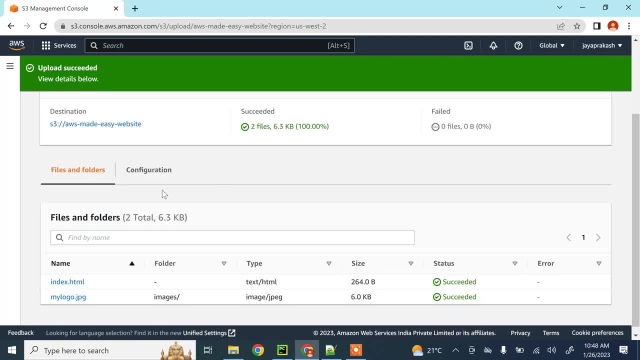 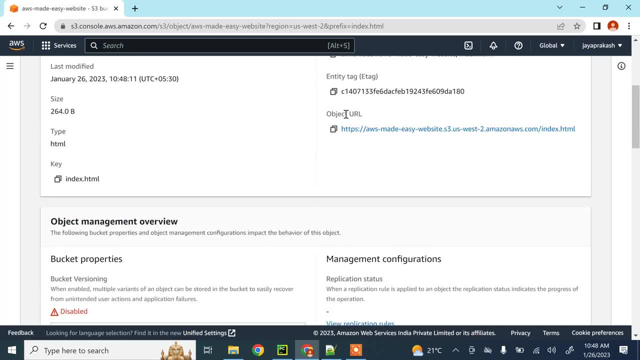 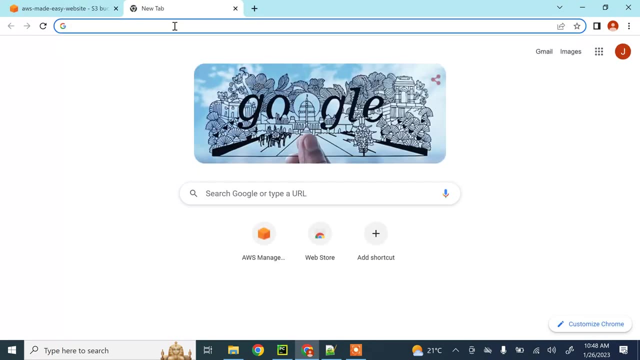 then I'm going to select add folder and select these images. Okay, Yep. So once you have uploaded these files, then you know you click on indexhtml. So this is the URL using which you will be able to access your website. So let's see now if you are able to access the website. So if you see it, 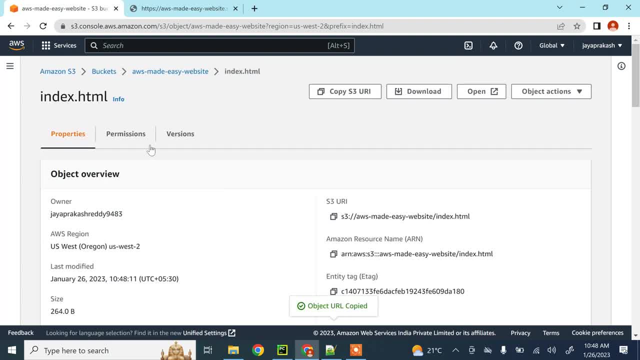 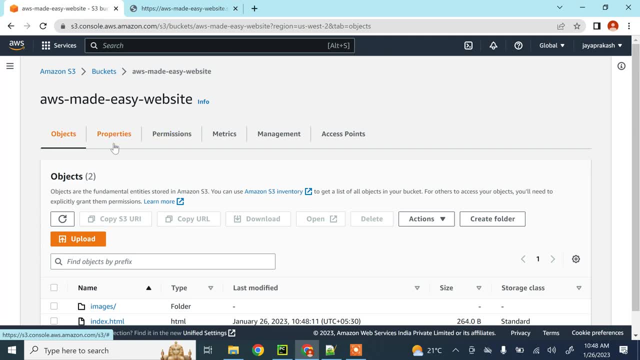 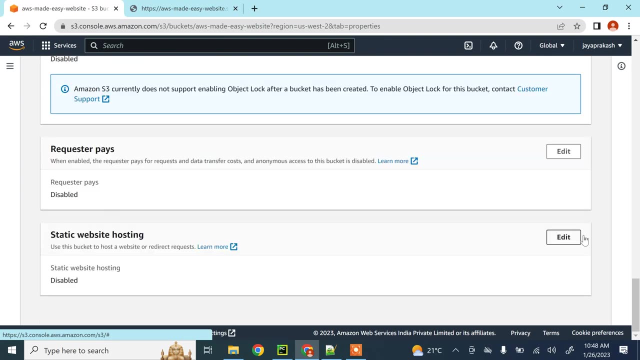 says that access denied. Okay, So now the first thing what we need to do is we need to make like: enable the static website hosting. So to do that, we click on properties here and scroll to the bottom. Here you see something called static website hosting. Click on edit here and enable the static website hosting and select this. 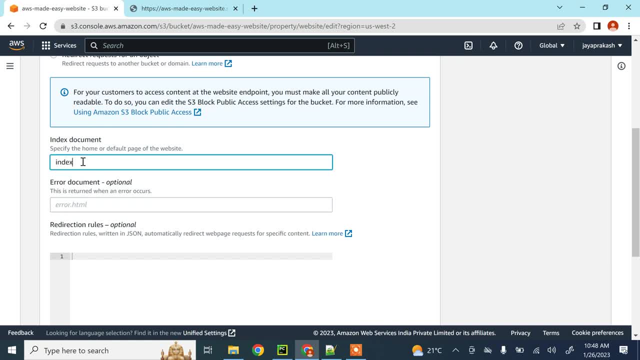 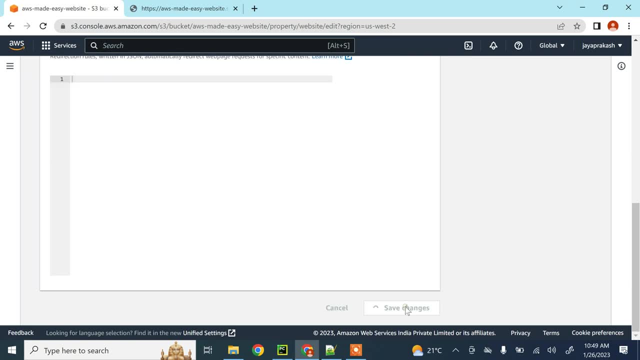 host a static website And you need to give the name of your index document. For me it is indexhtml. I'm going to leave this error document empty and click on save changes. Okay, So now let's see if you are able to access. 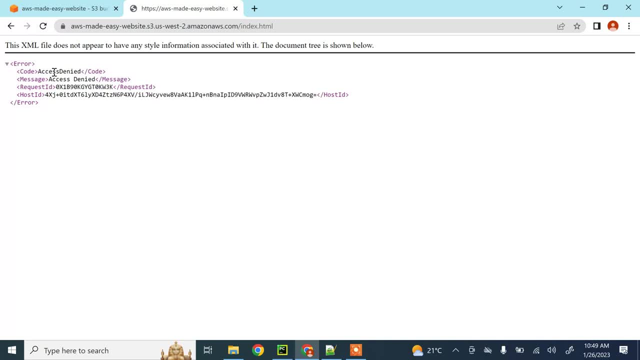 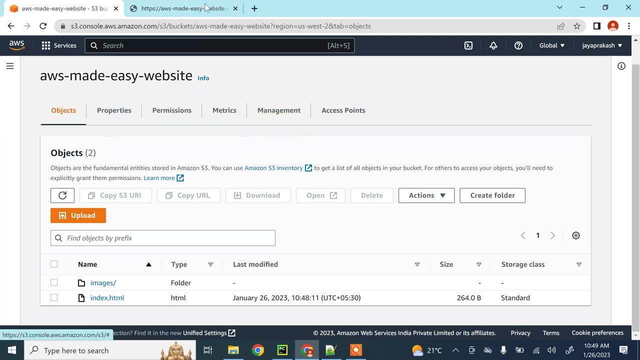 Okay, So I'm just going to refresh this. So, if you see again, we are seeing this access denied image, So access denied message, Okay, So what we need to do is we need to. basically, we are trying to access this website from internet, Right? So we need to make this bucket publicly accessible, Okay, So to 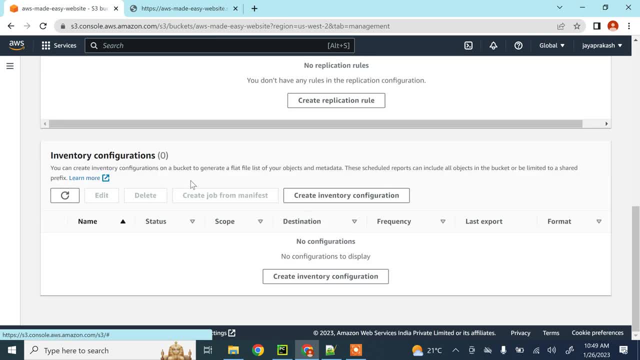 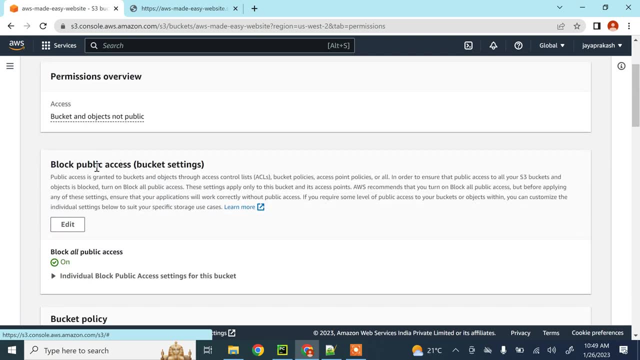 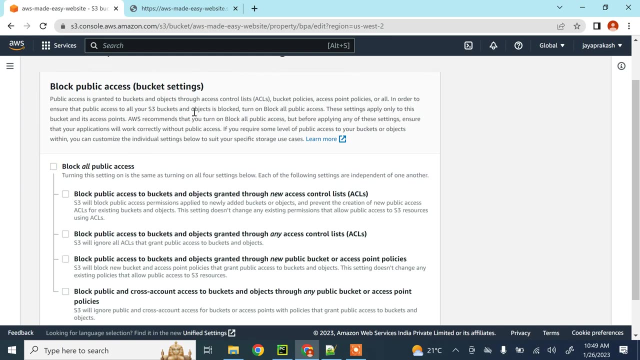 do that. I'm going to click on this management here- I'm sorry, permissions So- and click on block Public access here, Edit. So we need to uncheck this box. So what we are saying is we are saying, like AWS, to enable the public access to our S3 bucket. 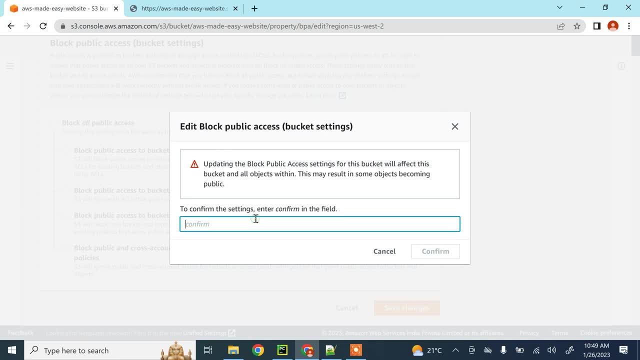 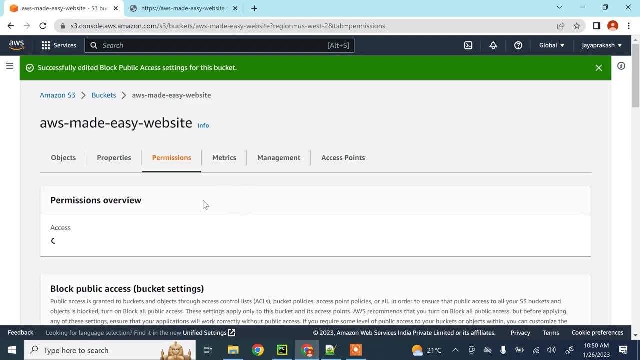 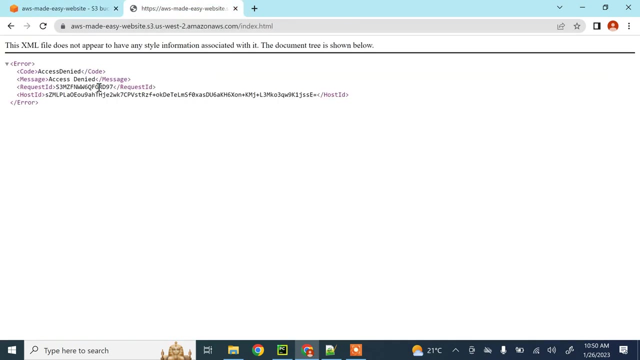 Okay. So I'm going to click on save changes here and type in confirm, Okay. So now let's see if you are able to access the website. So we are still seeing the access denied image. So what we need to do is: